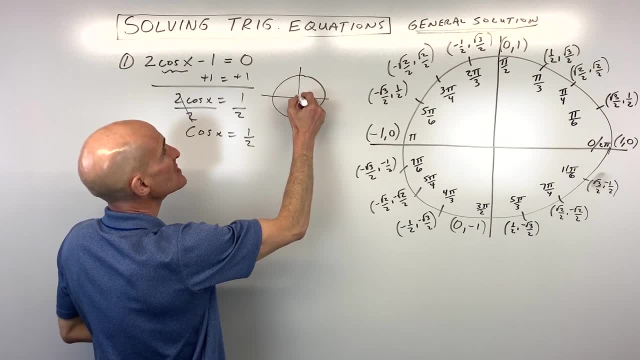 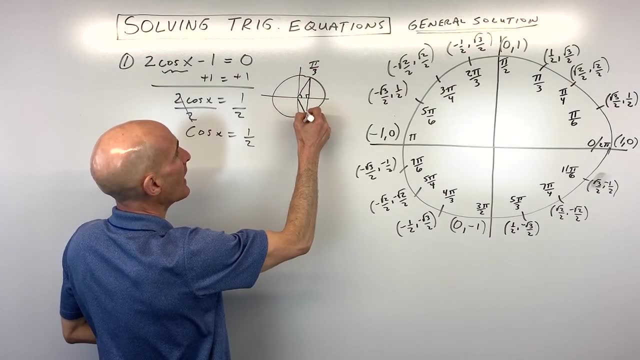 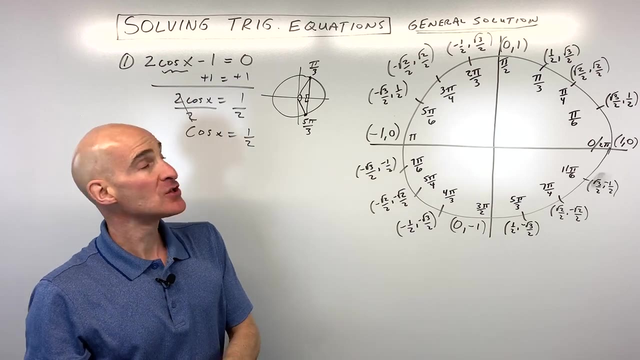 sketch over here just to illustrate. Here's our unit circle and you can see cosine's a half right here at pi over 3 or 60 degrees and over here at 5 pi over 3 or 300 degrees. Now notice these points here If we want to write a general. 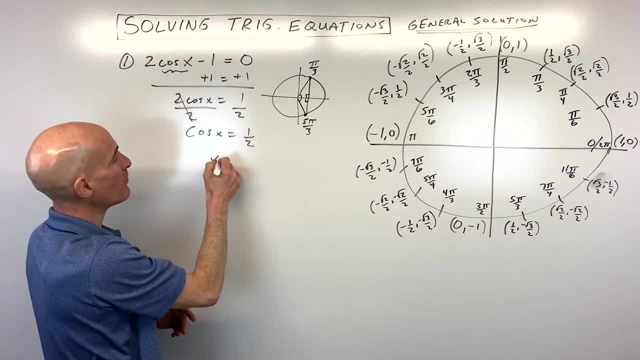 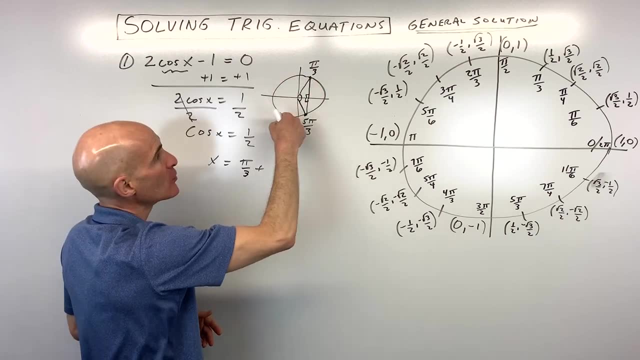 solution. what we have to do is we have to say x could equal pi over 3 plus if we add 2 pi or multiples of 2 pi, we're going to be going around that unit circle and we're going to be ending up in the same spot on the unit circle and 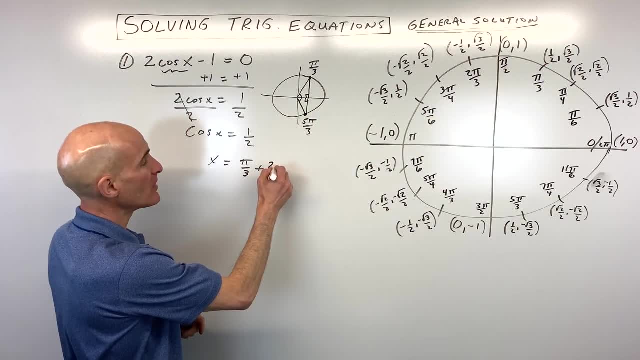 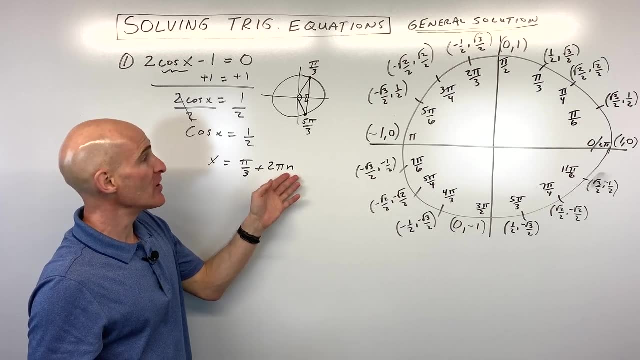 the value of the cosine is still going to be 1 half. So we're going to say pi over 3 plus 2 pi n, and then you can write where n is an integer meaning like n can't be a half or a third. You have to be multiples of 2 pi. You know it can be. 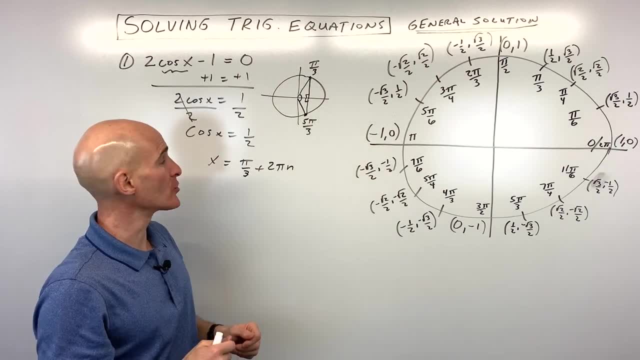 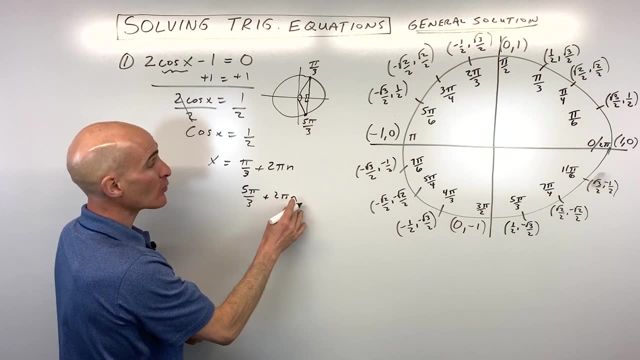 positive or negative. You can go either direction around the unit circle, So it can also be 5 pi over 3 plus 2 pi n, again where n is an integer. So this is our general solution for the answer to this equation. Now we're going to go into a little bit more. 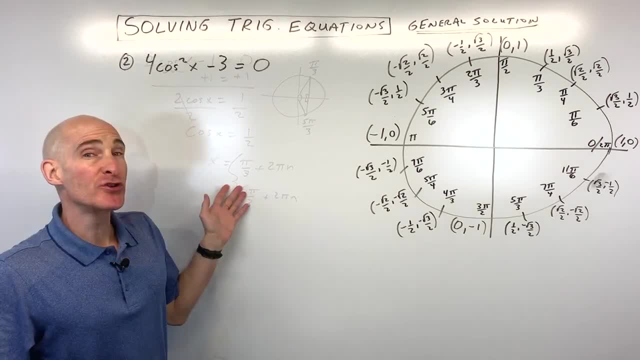 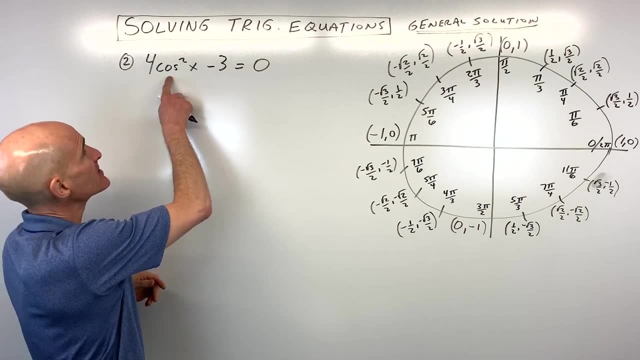 challenging one in the next example. so let's dive into that one. next, Okay, number two, see if you can do this one. We have 4 cosine squared of x minus 3 equals 0. So again, we're trying to isolate that trig function by itself on one side of. 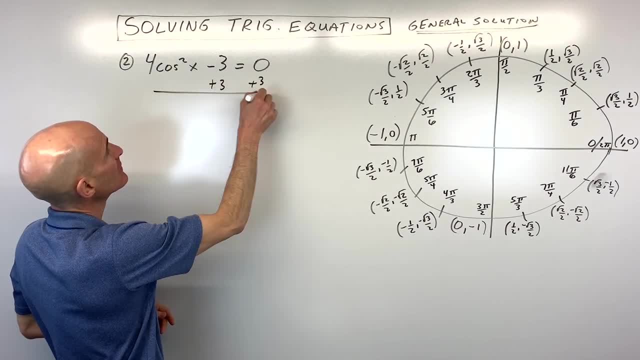 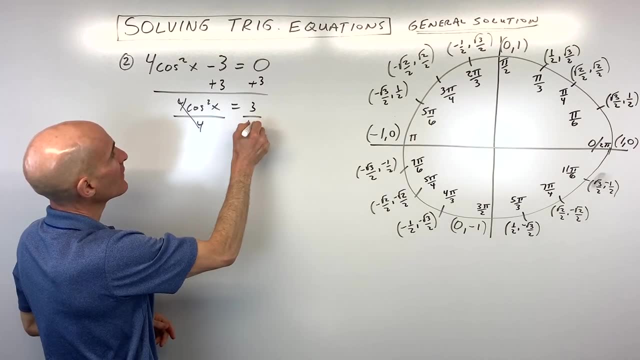 the equation. So we're going to add 3 to both sides, So we get 4. cosine squared of x is equal to 3.. We're going to divide both sides by 4 and now we have cosine squared of x equals 3 fourths. What we're going to want to do is take the square root of both. 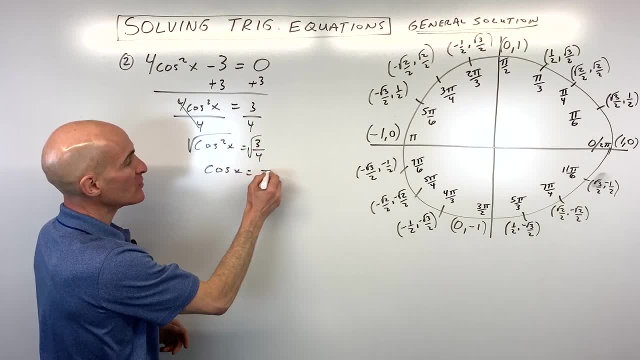 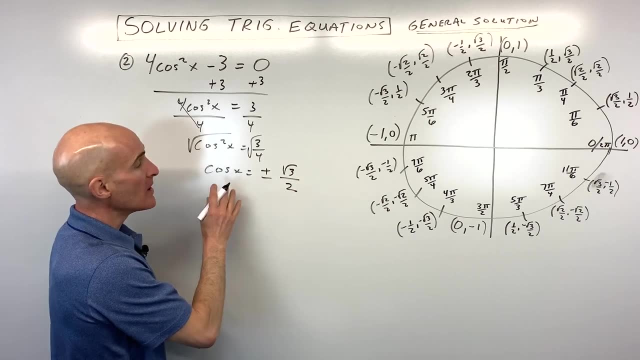 sides to get the cosine by itself. And when we do that, when you take the square root of both sides, you get two answers: positive or negative. Square root of 3 we're going to leave as square root of 3.. Square root of 4 is equal to 2.. So now what we're doing. 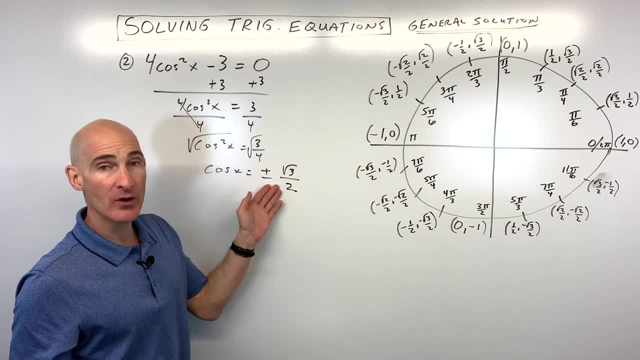 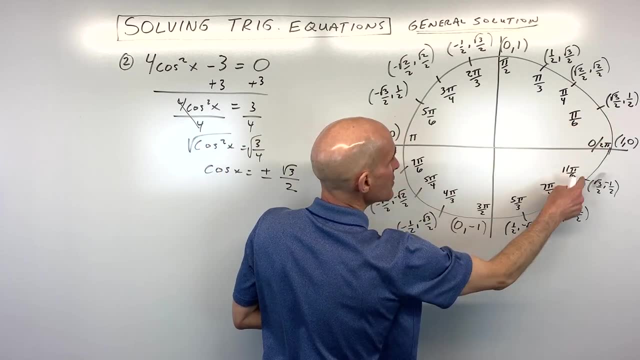 is we're saying cosine of what angle equals positive root of 3 over 2 or negative root of 3 over 2.. And remember, the cosine is the x coordinate on the unit circle. So you can see it's going to be positive root of 3 over 2 here and here Negative root of 3 over 2. 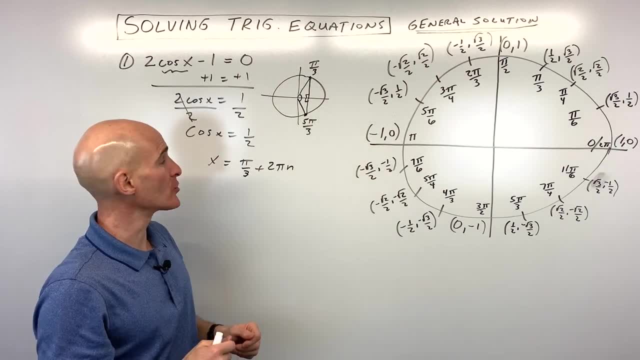 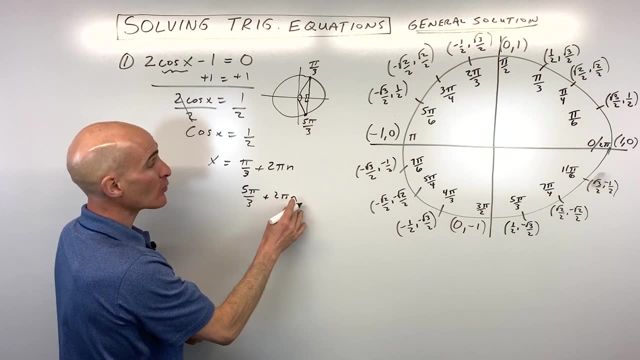 positive or negative. You can go either direction around the unit circle, So it can also be 5 pi over 3 plus 2 pi n, again where n is an integer. So this is our general solution for the answer to this equation. Now we're going to go into a little bit more. 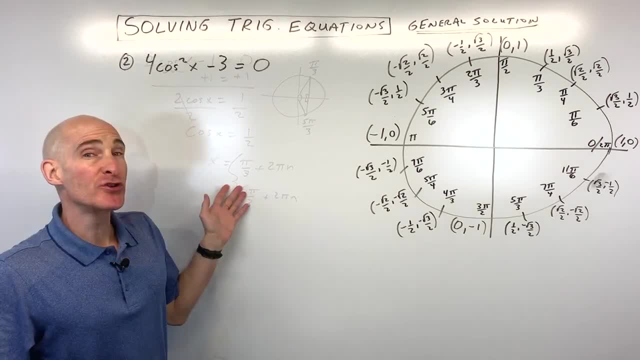 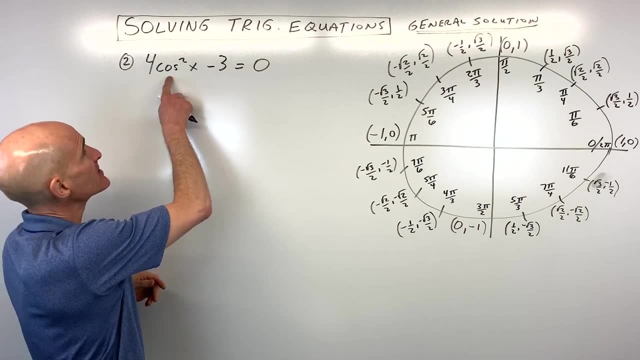 challenging one in the next example. so let's dive into that one. next, Okay, number two, see if you can do this one. We have 4 cosine squared of x minus 3 equals 0. So again, we're trying to isolate that trig function by itself on one side of. 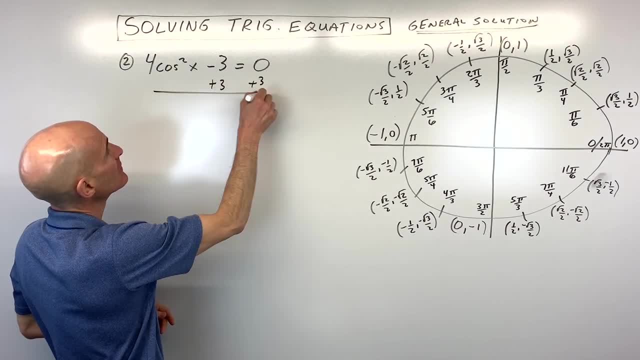 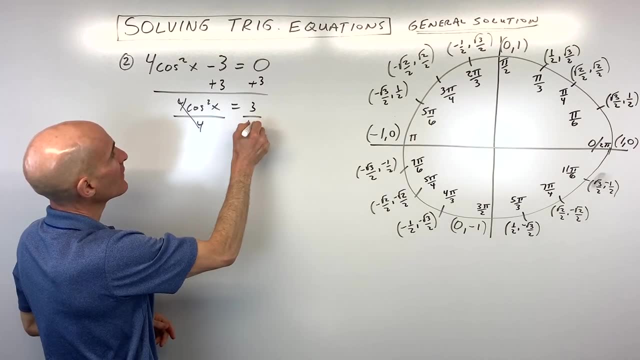 the equation. So we're going to add 3 to both sides, So we get 4. cosine squared of x is equal to 3.. We're going to divide both sides by 4 and now we have cosine squared of x equals 3 fourths. What we're going to want to do is take the square root of both. 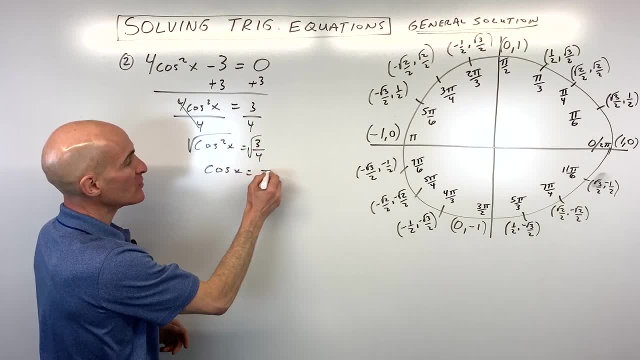 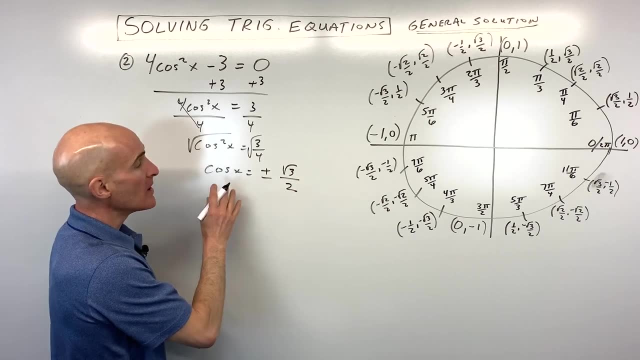 sides to get the cosine by itself. And when we do that, when you take the square root of both sides, you get two answers: positive or negative. Square root of 3 we're going to leave as square root of 3.. Square root of 4 is equal to 2.. So now what we're doing. 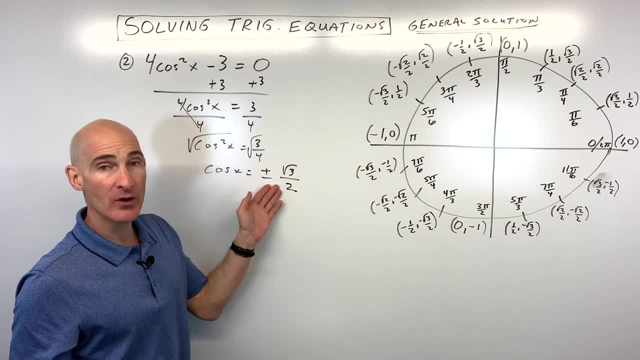 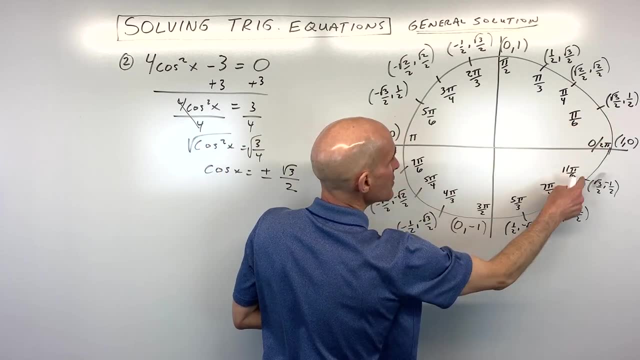 is we're saying cosine of what angle equals positive root of 3 over 2 or negative root of 3 over 2.. And remember, the cosine is the x coordinate on the unit circle. So you can see it's going to be positive root of 3 over 2 here and here Negative root of 3 over 2. 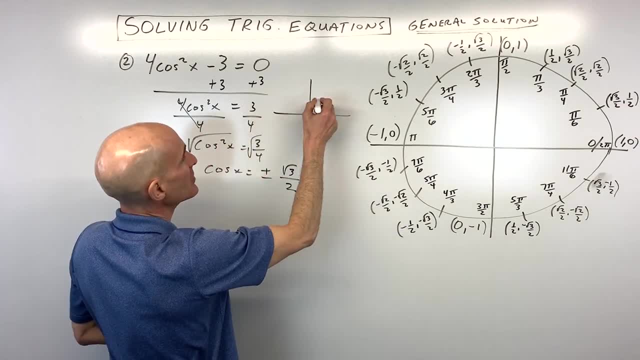 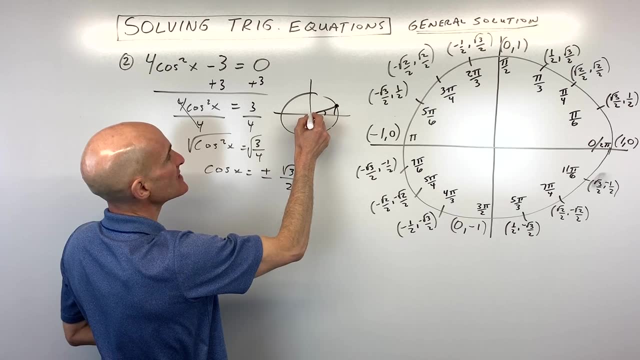 here and here. So if I just draw a sketch just to kind of illustrate here, you can see we're at these 30 degree angles, these pi over 6 degree reference angles. So you can see it's actually going to be pi over 6 in each of these quadrants: first, second, third and fourth. But what? 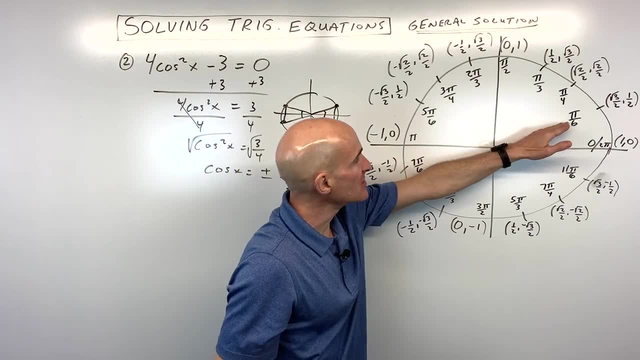 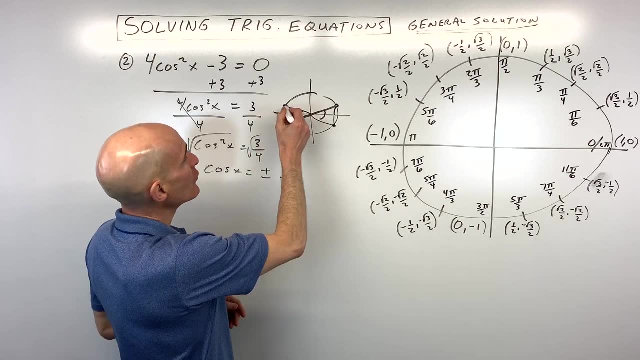 I want you to notice is that see how over here, at pi over 6 and 7 pi over 6, see how they're like diametrically opposed. It's like a diameter like across from each other. And same thing over here with 5 pi over 6 and 11 pi over 6.. These ones are diagonally. 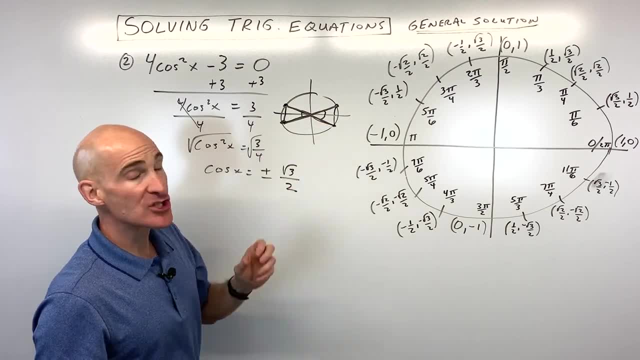 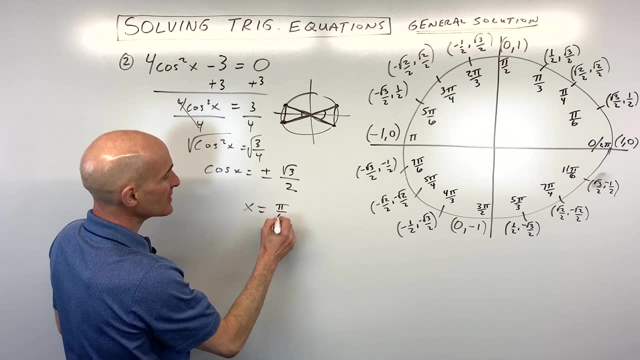 opposed. They're across from each other, diametrically opposed. So we write our general solution. we can group those together to make it a little bit more compact of an answer. So we have x equals pi over 6 plus, because we're going halfway around the circle here. that represents: 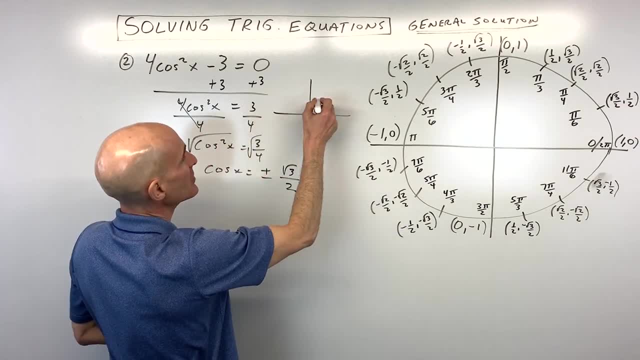 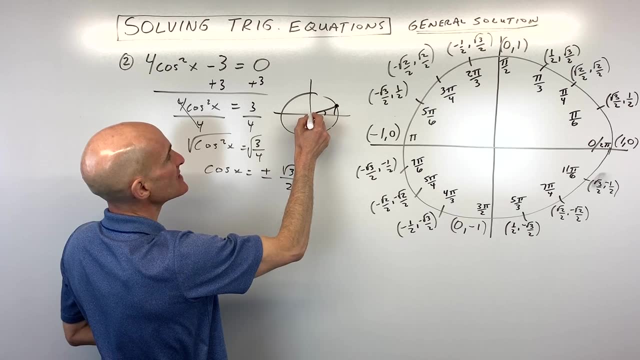 here and here. So if I just draw a sketch just to kind of illustrate here, you can see we're at these 30 degree angles, these pi over 6 degree reference angles. So you can see it's actually going to be pi over 6 in each of these quadrants: first, second, third and fourth. But what? 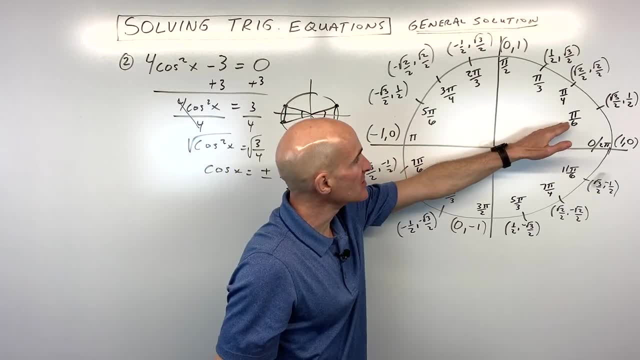 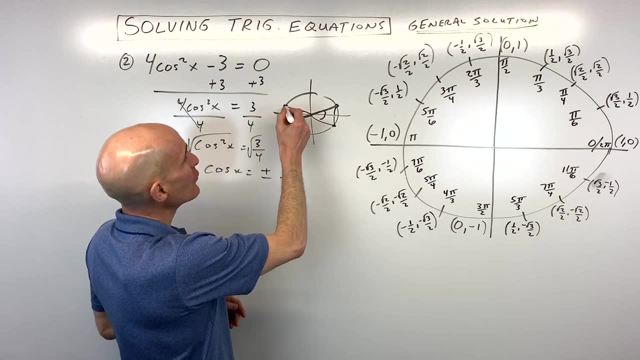 I want you to notice is that see how over here, at pi over 6 and 7 pi over 6, see how they're like diametrically opposed. It's like a diameter like across from each other. And same thing over here with 5 pi over 6 and 11 pi over 6.. These ones are diagonally. 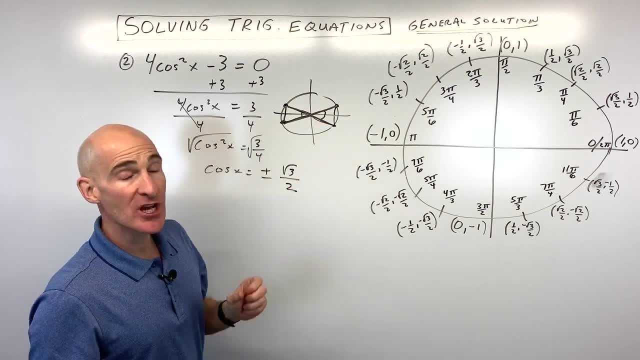 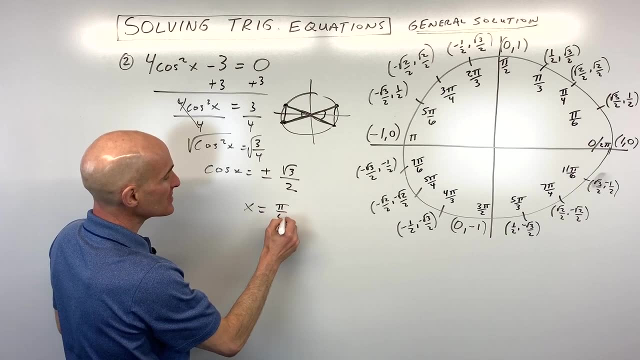 across from each other diametrically opposed. So when we write our general solution we can group those together to make it a little bit more compact of an answer. So we have x equals pi over 6 plus, because we're going halfway around the circle here. that represents: 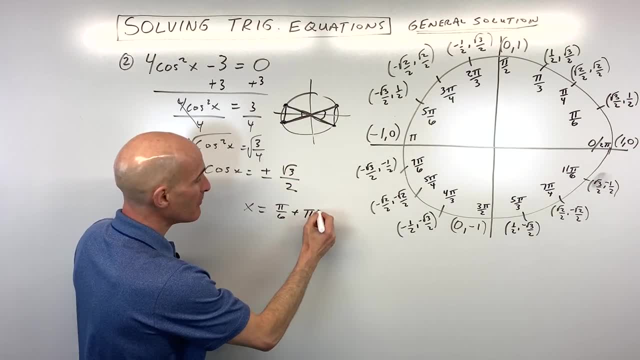 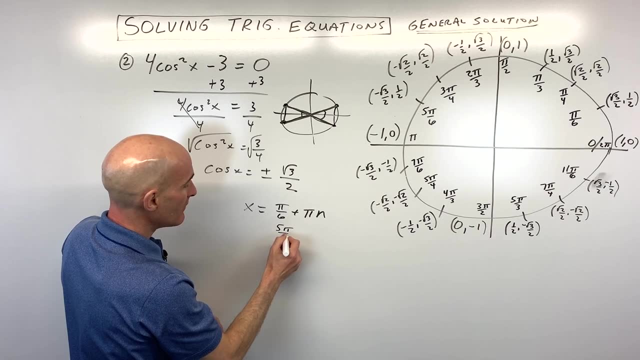 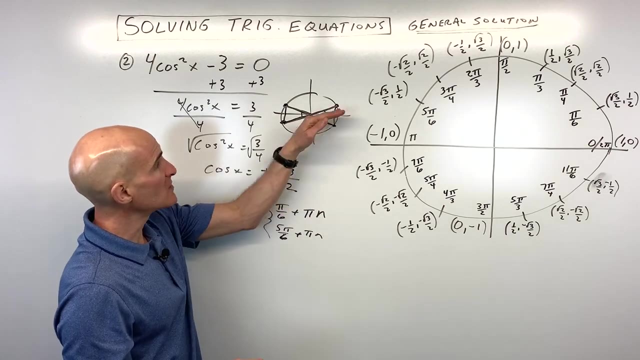 180 degrees or pi radians. So we're going to say plus pi n where n is an integer. And also we're going to take this one here: 5 pi over 6 plus pi n where n is an integer, a half, a third, etc. So we were able to group these together to make it a little bit more compact. 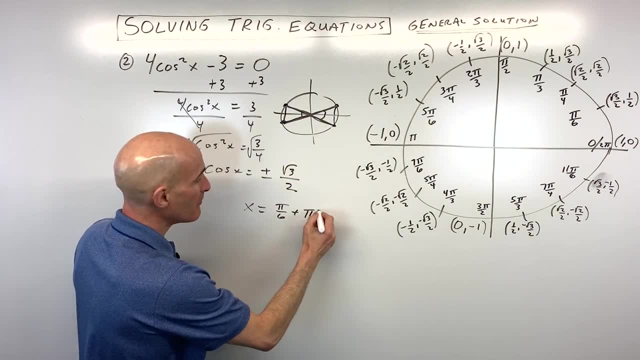 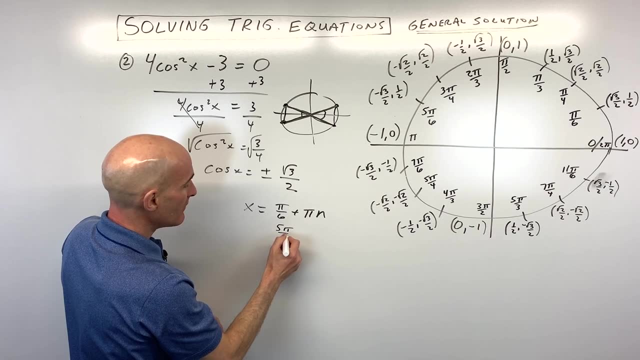 180 degrees or pi radians. So we're going to say plus pi n, where n is an integer. And also we're going to take this one here: 5 pi over 6,, 5 pi over 6, plus pi n, where n. 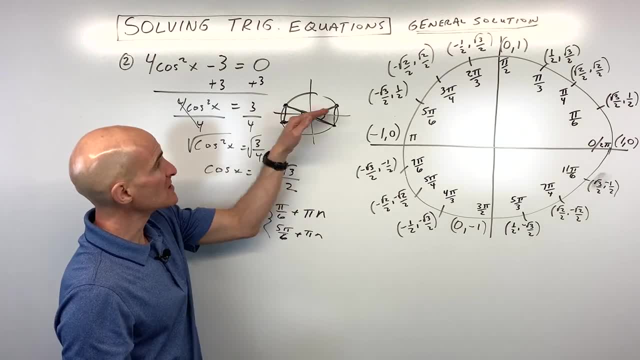 is an integer, It can't be pi n, 5, pi over 6 plus pi n. where n is an integer, It can't be a half, a third, etc. So we were able to group these together to make it a little bit more. 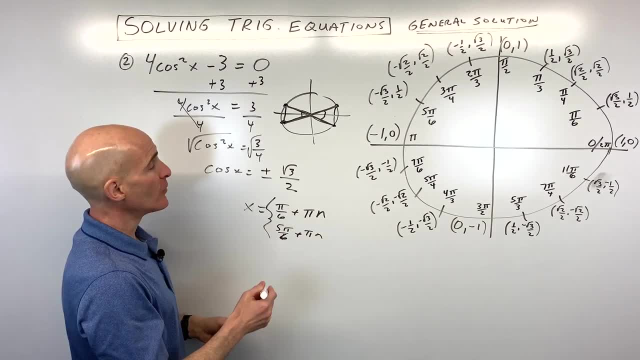 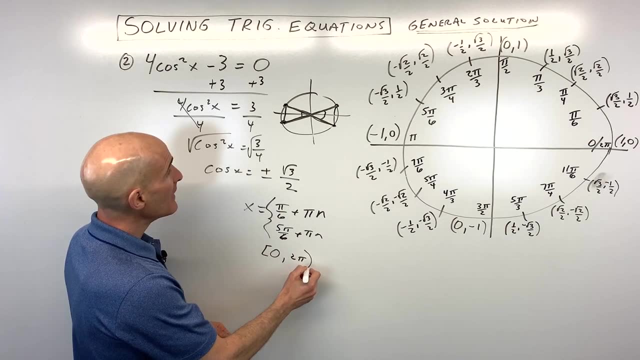 compact. This would be our general solution. If it just said: you know, find all the solutions between 0 to 2 pi. okay, like this, then you would just say: pi over 6,, 5, pi over 6,, 7, pi over 6, and 11 pi. 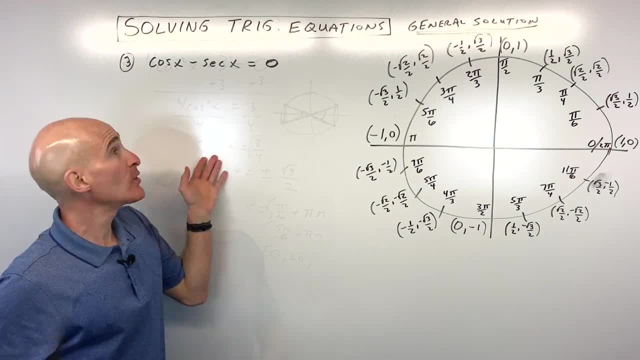 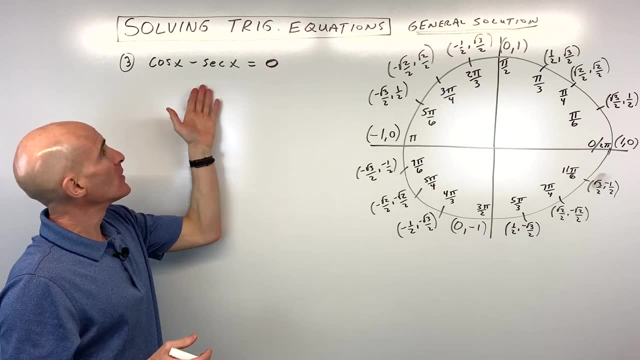 over 6.. But what we're focusing on here is writing a general solution. Okay, number three: we have a little bit more challenging one. We have cosine x minus secant of x equals 0. How do we solve that one? And, by the way, if you like the way that I'm explaining these concepts and you want to go, 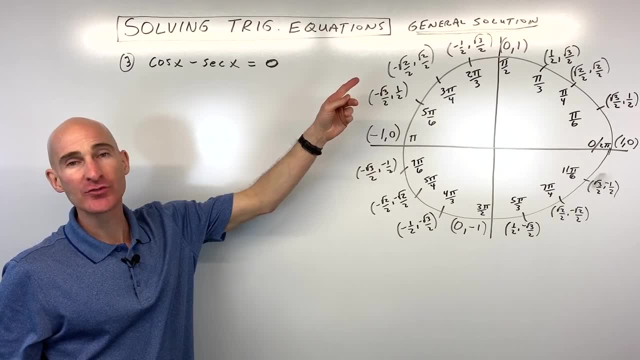 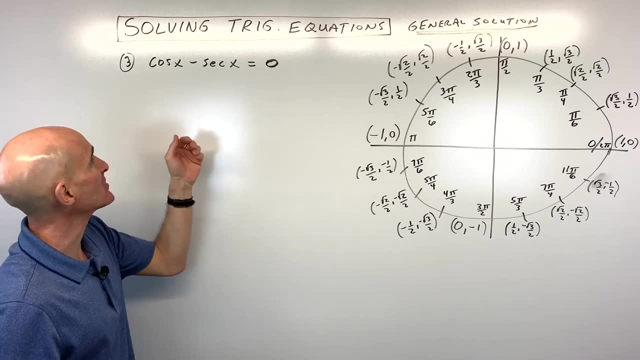 deeper into algebra 2, definitely check out my algebra 2 video course for sale that goes into all these different concepts plus more covering algebra 2 topics. But let's jump into this one here. What we're going to do is we're going to change the secant of x into 1 over cosine of x. 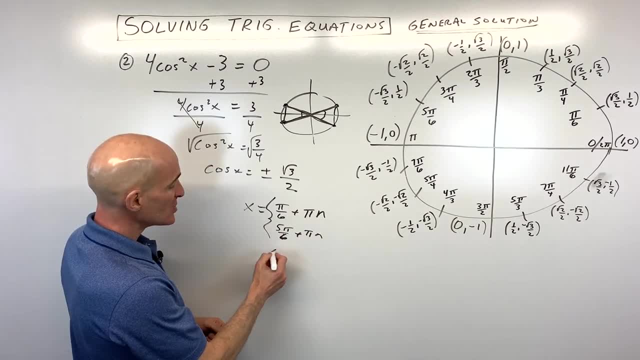 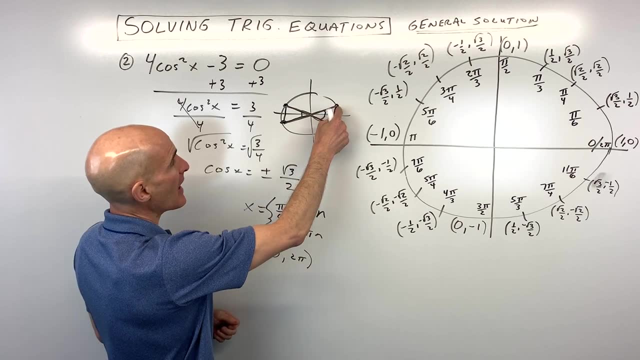 This would be our general solution. If it just said: you know, find all the solutions between zero to two pi. okay, like this, then you would just say pi over six, five pi over six, seven pi over six and eleven pi over six. But what we're focusing on here is writing a general solution. 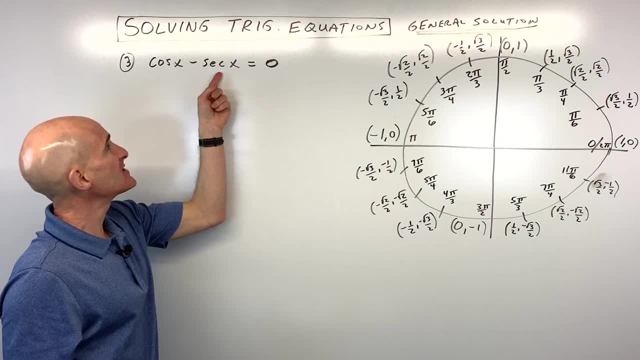 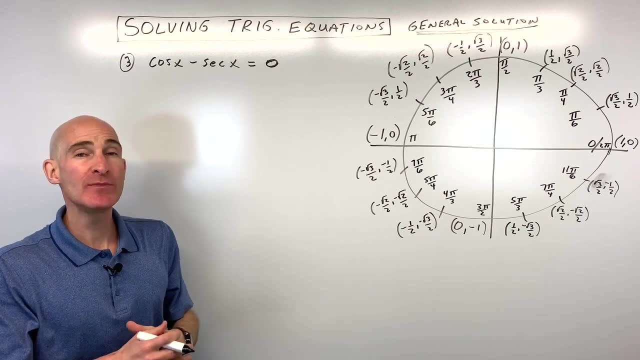 Okay, number three. we have a little bit more challenging one. We have cosine x minus secant of x equals zero. How do we solve that one? And, by the way, if you like the way that I'm explaining these concepts and you want to go deeper into algebra two, definitely check out my algebra two. 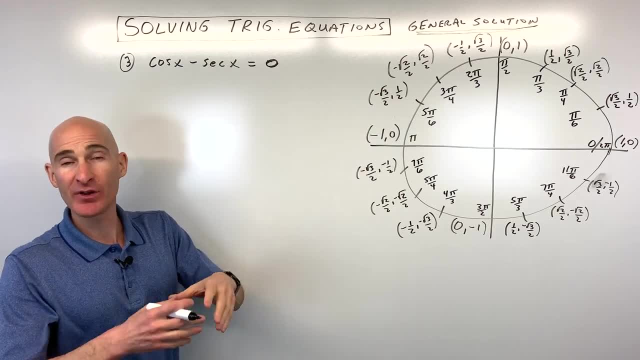 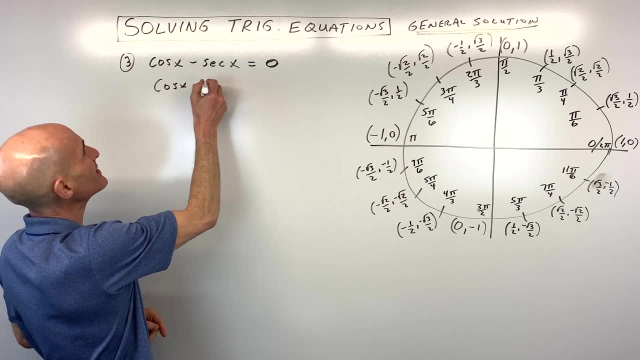 video course for sale that goes into all these different concepts plus more covering algebra- two topics, But let's jump into this one Here. what we're going to do is we're going to change the secant of x into one over cosine of x because, remember, secant is a reciprocal of cosine, right? 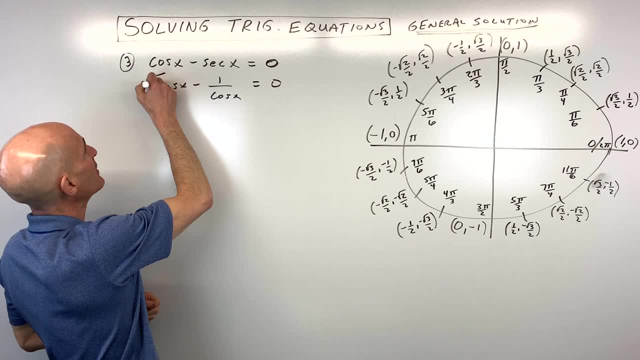 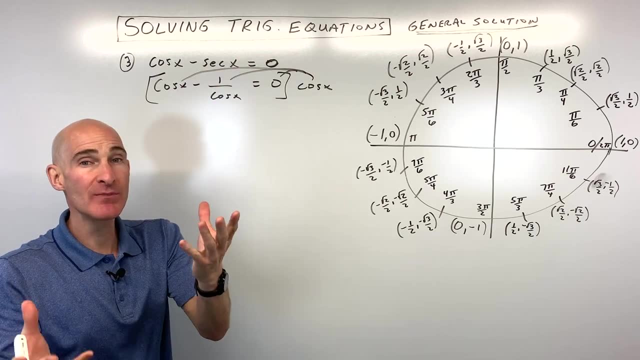 And so now what we're going to do is we're going to clear this denominator here by multiplying through by the cosine of x. So I'm going to distribute that cosine, Cosine of x, to the left and right sides of the equation, keeping it balanced right. 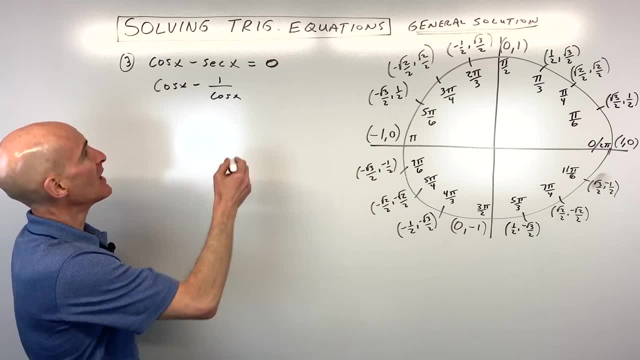 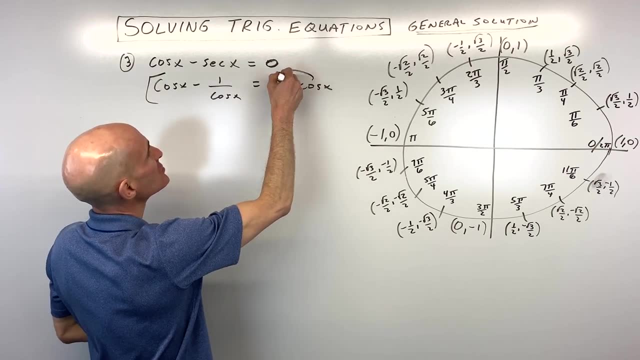 because, remember, secant is a reciprocal of cosine right. And so now what we're going to do is we're going to clear this denominator here by multiplying through by the cosine of x. So I'm going to distribute that cosine of x to the left and right sides of 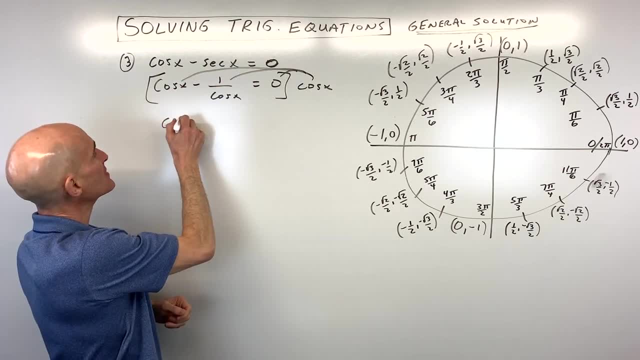 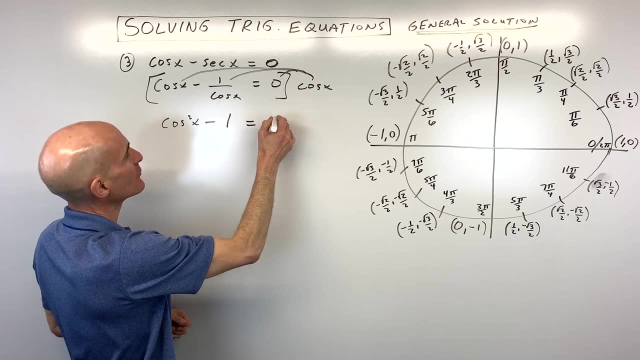 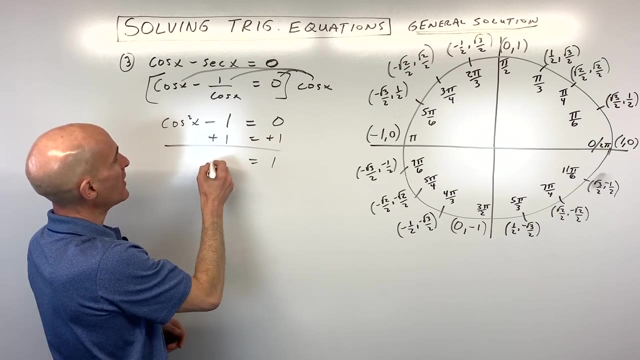 the equation, keeping it balanced right. So this is going to give us cosine squared of x minus 1, okay, because here these are canceling numerator and denominator and 0 times anything, of course, is 0. So now I'm going to add 1 to both sides of the equation. So this gives us 1 and cosine. 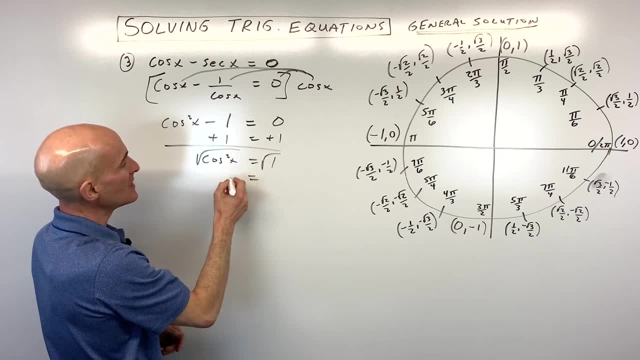 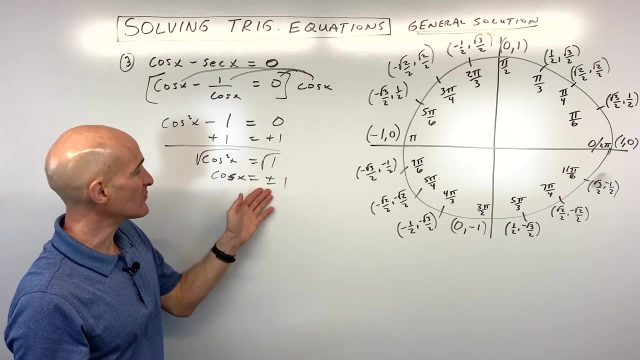 squared x. And if we take the square root now of both sides to get the cosine by itself, we get plus or minus 1, because, remember, when we take the square root of both sides we get those two answers: positive or negative. So now we go to the unit circle. Remember, cosine is the x. 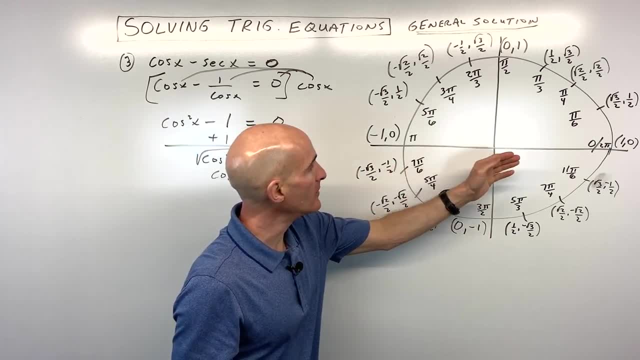 coordinate on the unit circle And we say, well, where is the x coordinate? 1 or negative 1? So it's going to be 1 here and it's going to be negative 1 here, And those are the only two locations. So